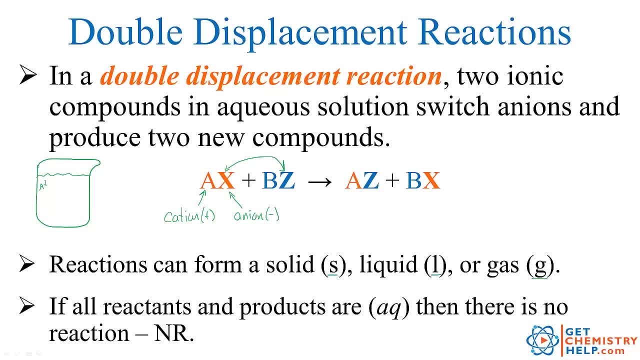 So I dissolve those up and they're soluble. So I've got my a cations swimming around in here and I've got my x anions and they're swimming around And then I dissolve up bz. so I've got b cations swimming around in here. 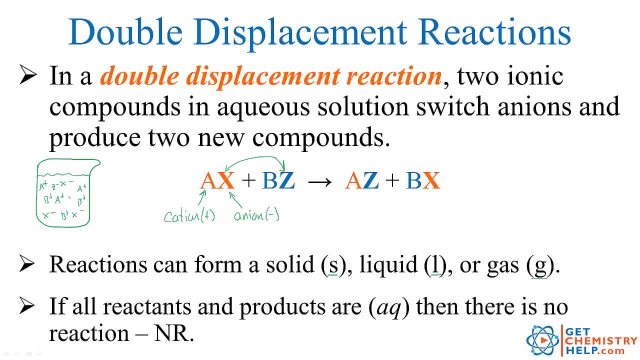 and then I've got z anions. So here's my z anions. Okay, so a and x and b and z are all dissolved and they're just swimming around. Well, if, once the reaction is done and they've all mixed together and they're still just swimming around, if no solid is formed, no liquid is formed, no gas is formed. 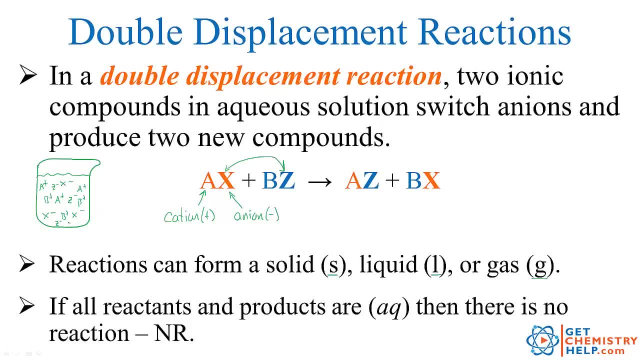 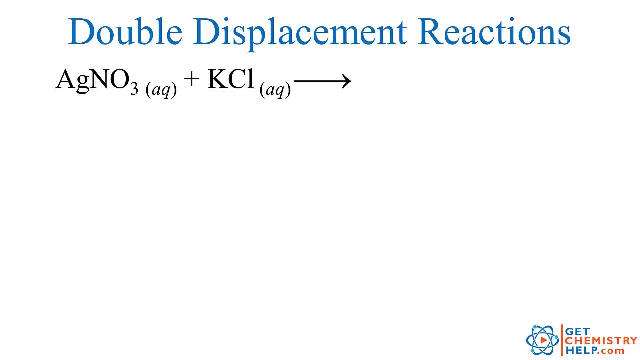 then really nothing happened. We would just write nr, so instead we would just write n. So let me show you an example here. So silver nitrate combines with potassium chloride. So this is silver nitrate, kCl is potassium chloride. well, silver was with nitrate, potassium was with chloride. 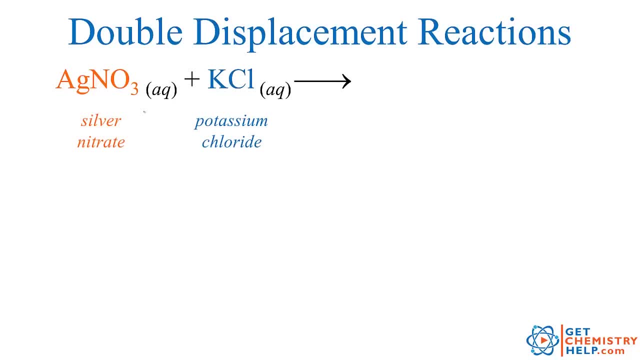 Basically, we just swap partners, so silver nitrate with potassium chloride, And after that we're left with the question to how do I rank this? So that's what I'm going to be: TW union: Silver goes with chloride and potassium goes with nitrate. 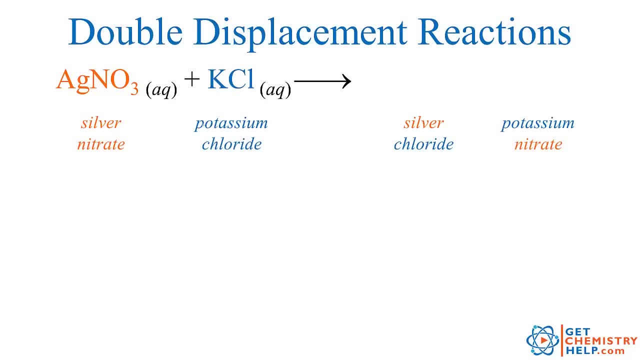 So we think of it as making silver chloride and potassium nitrate. Now we can figure out what the formula for silver chloride and potassium nitrate are. So silver chloride is AgCl, potassium nitrate is KNO3.. And our last step is to figure out. well, what is the physical state on this? 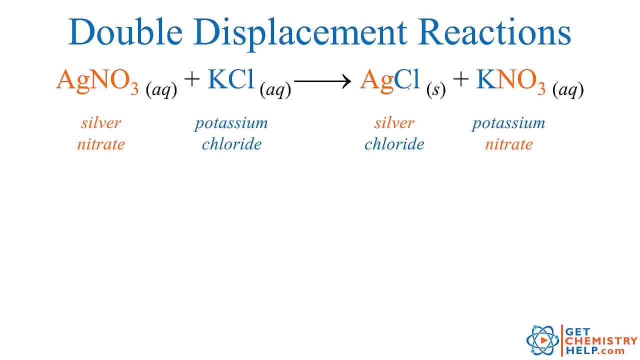 Is it aqueous, solid, liquid or gas? So silver chloride is a solid. potassium nitrate is aqueous. Well, the question, of course, is how in the world do you know this? Well, there are some solubility rules that summarize the solubility of different ionic. 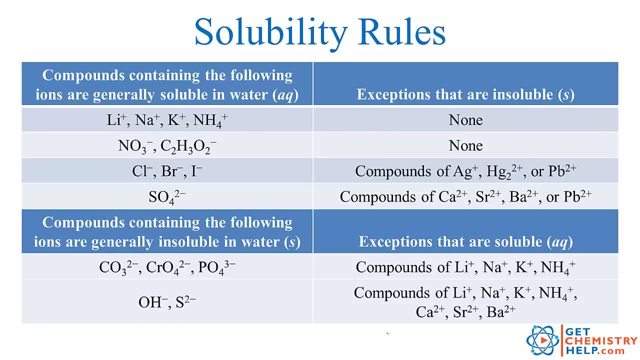 compounds based on what ions they contain. Now, if you follow this link down below to GetChemistryHelpcom, you can print out a PDF that has all of these solubility rules summarized on it. But generally the way it works is compounds that contain the following ions: 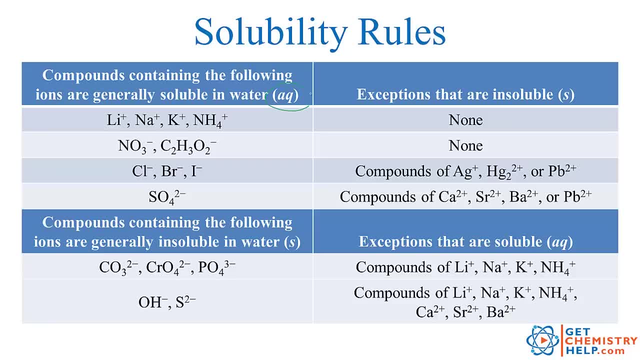 Ions are generally soluble in water. that means they are aqueous. So if you have an ionic compound and it has any of these ions- lithium, sodium, potassium, ammonium nitrate, acetate, chloride, bromide, iodide, sulfate- they are generally always. 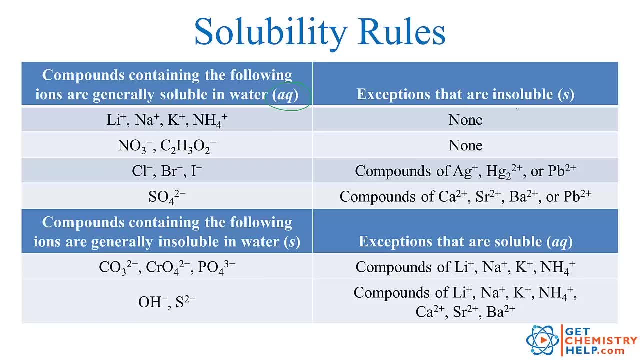 going to be soluble or aqueous. Now notice, there are a few exceptions, though, that are solids, So lithium, sodium, potassium, ammonium. these don't have any exceptions, Those are always aqueous. Any nitrate compound or acetate compound. 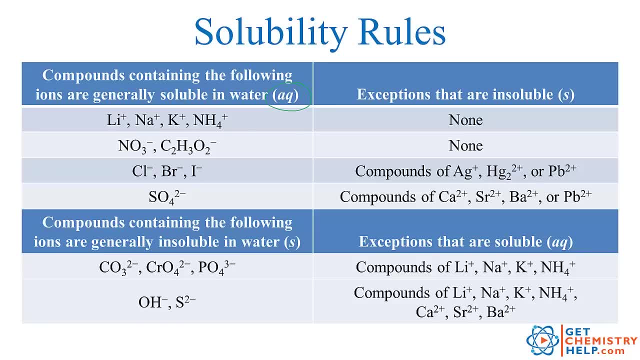 Almost all of them are aqueous, Almost always aqueous, No exceptions. Chlorides, bromides, iodides, any of those ionic compounds are also aqueous, But there are a few exceptions. So if you had silver, mercury 1 or lead combined with chloride bromide iodide, those would 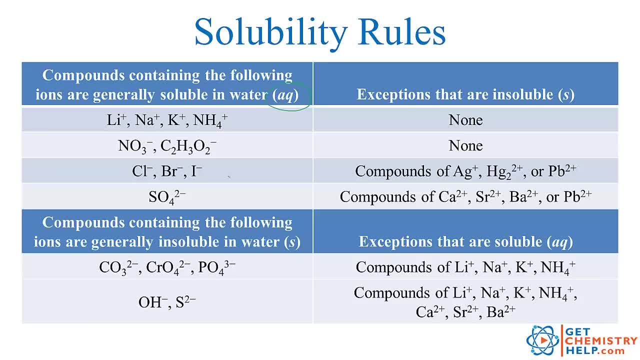 be solid, but every other chloride, bromide and iodide would be aqueous. How about sulfate? All sulfates are aqueous unless it's calcium sulfate, strontium sulfate, barium sulfate or lead 2 sulfate. Now the bottom half of the table tells you which types of ions are going to be solid. 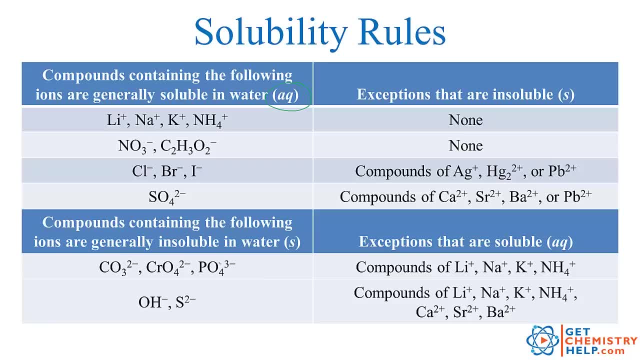 or insoluble. So anything with carbonate, chromate or phosphate is a solid, except, of course, we said, anything with lithium. sodium, potassium and ammonium are always soluble. So even with these, if it has lithium, sodium, potassium or ammonium, those are all soluble. 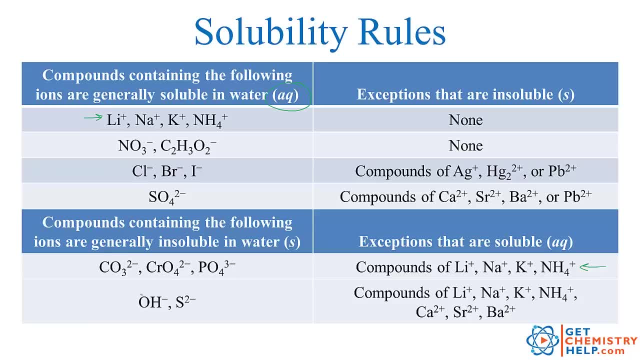 But any other carbonate, chromate or phosphate would be a solid, Same with hydroxide or sulfide. These are always solids, except again with lithium, sodium, potassium or ammonium, but also if they're with calcium, strontium or barium. 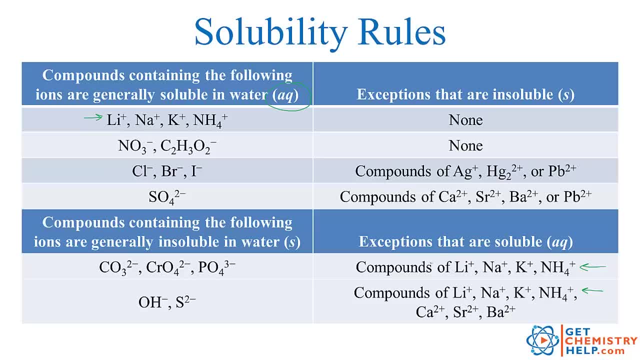 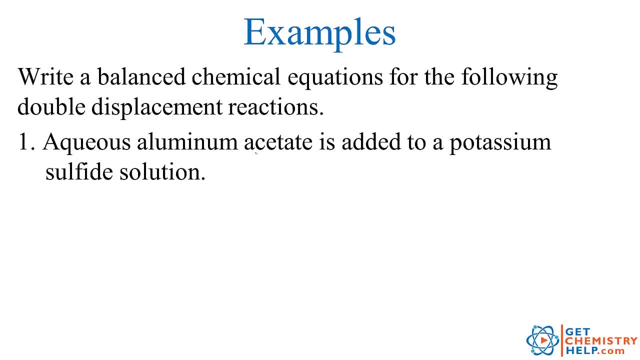 So calcium, strontium or barium hydroxide or sulfide would also be soluble, But all other hydroxides and sulfides would be solids. Okay, so let's try a few examples of these. So it tells me to write a balanced chemical equation for the following double displacement: 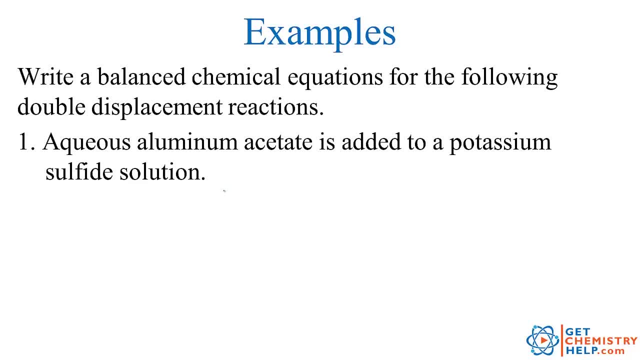 reactions. Now again, it would be convenient for you to have those solubility rules handy So you can go to GetChemistryHelpcom and print those out and have those here in front of you. So aqueous aluminum acetate is added to a potassium sulfide solution. 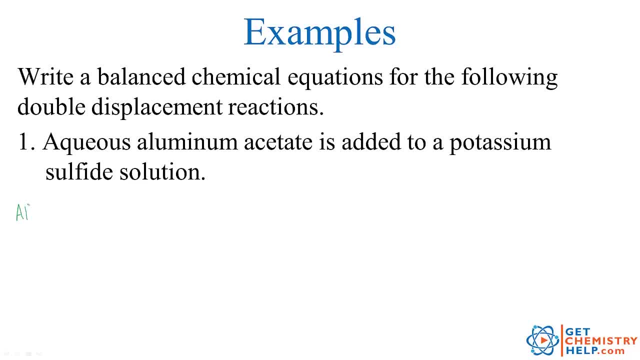 Okay, aqueous aluminum acetate. well, we know from our lessons on naming that aluminum is three positive. acetate is C2H3O2 negative. So aluminum acetate would combine and make Al parentheses C2H3O2.. Okay. 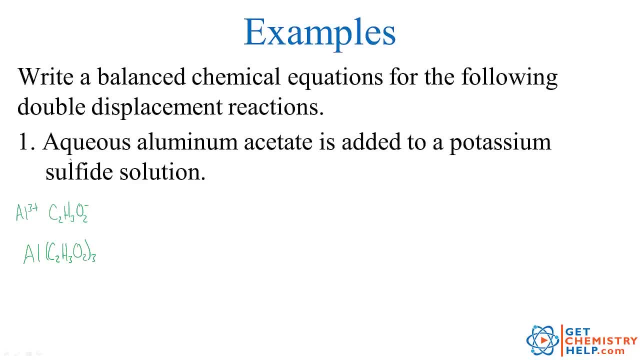 Okay, So C2H3O2, parentheses three, And it already told us it was aqueous. If you look at your solubility rules, you can see that anything that has acetate is always soluble Aqueous. Does that make sense? 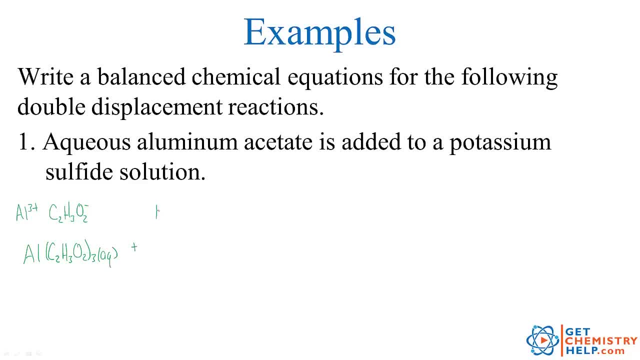 That's added to potassium sulfide. Well, potassium is positive, sulfide is two negative. So that would make K2S. And again, if you look at your solubility rules, anything with potassium is soluble, So that's why it's a solution. 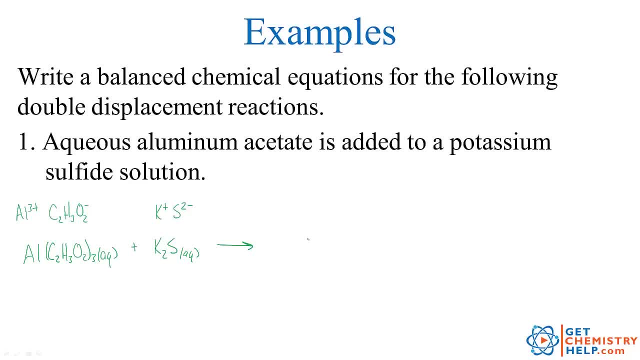 So aqueous. Now we're going to predict our products. Well, the wrong way to try to predict the products is just to try to keep the same ratio as the ions originally had. So you can't say: originally it was one aluminum and one sulfide, so aluminum, sulfide must. 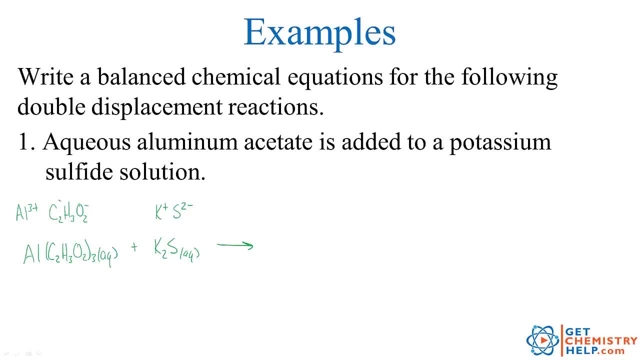 be one of each. You can't do that. You have to figure it out based off the charges. So now aluminum is partnering up with sulfide. So aluminum three positive, combining with sulfide two negative, What would that be? Well, that would be Al2S3.. 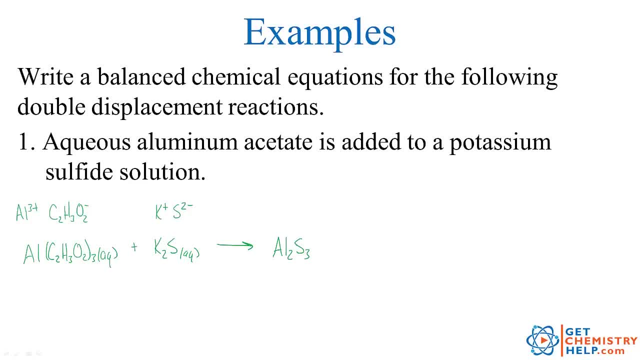 If you look on your solubility rules, you'll see all sulfides are solids, insoluble except for a few exceptions, And aluminum is not one of those. So this is a solid. Then we're also going to combine potassium with acetate. 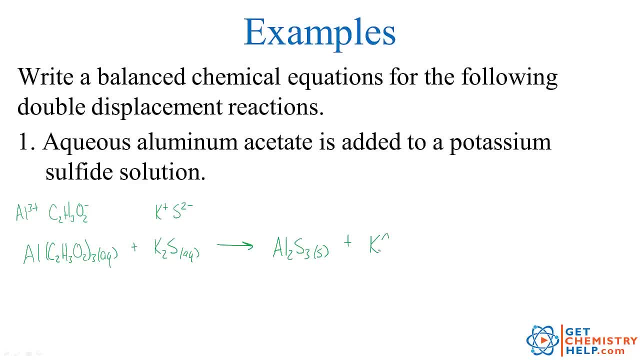 Well, that's K positive, acetate negative, So just one of each will make a neutral compound. And if you look on your solubility rules, All potassium containing compounds are soluble. All acetate containing compounds are soluble, So this is definitely aqueous. 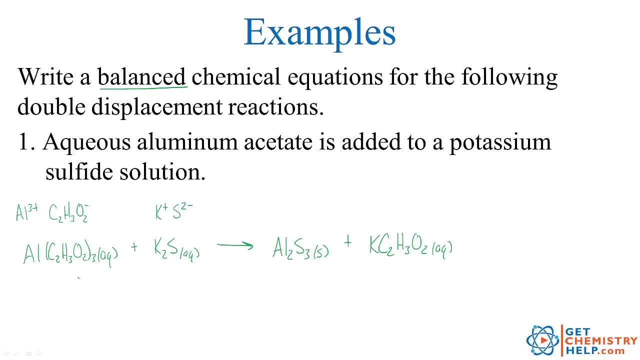 Well, the last thing we have to do is to balance it, So we'll just go through and use our balancing skills. First off, we're going to identify that there is a polyatomic on both sides, So I'll balance this as one unit. 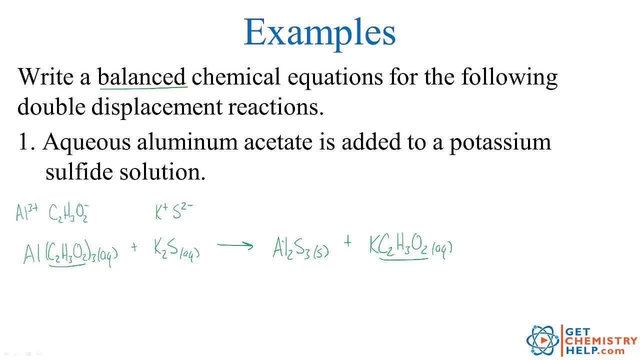 So one aluminum on the reactants, two aluminums on the products. So let's make this two aluminums. Now I've got two times three: Six acetates on the reactants, Only one acetate on the product, So we need to make that into a six. 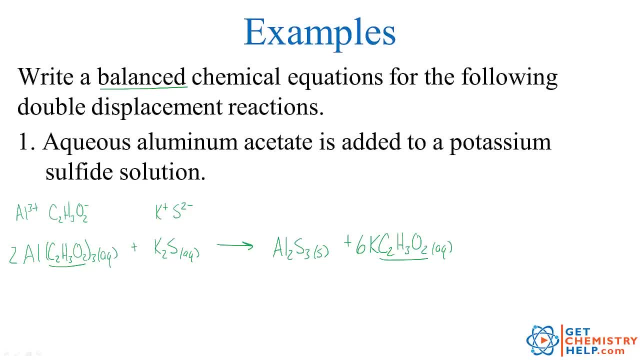 Well, as soon as I do that, that also makes six potassiums. So we need six potassiums on the reactants. So here's two. So in order to make two into six, I've got to multiply it by three. Well, now I've got three sulfides. 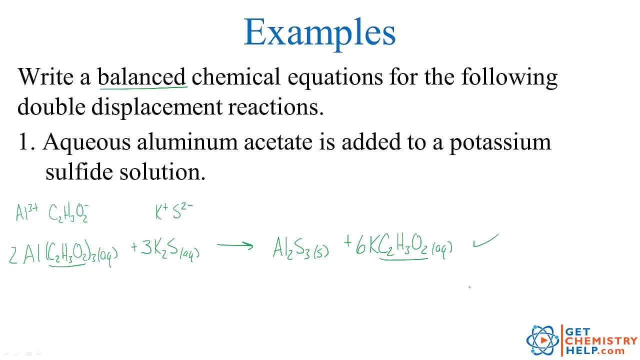 And this has three sulfides. So there you go. This reaction is balanced, Looks good. Number two: Aqueous barium chloride Is added to a sodium carbonate solution. Well, barium is two positive, Chloride is Cl negative. 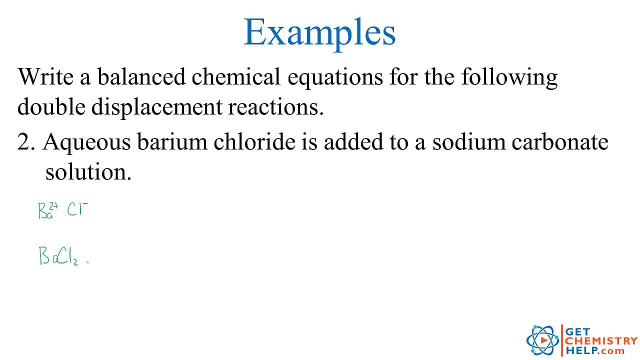 So that would be BaCl2.. And all chlorides are soluble except silver, mercury and lead, So that would be soluble. Is added to sodium carbonate, So sodium is Na positive, Carbonate is CO3 two negative, So that would make Na2CO3. 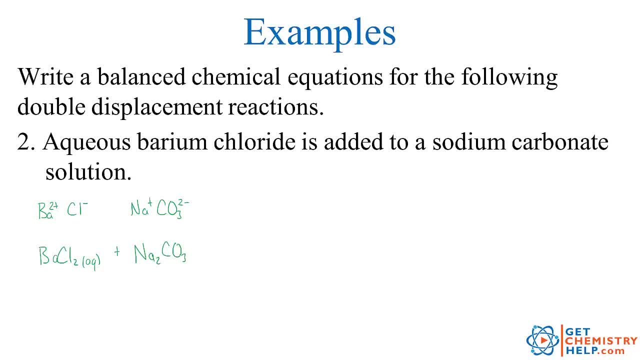 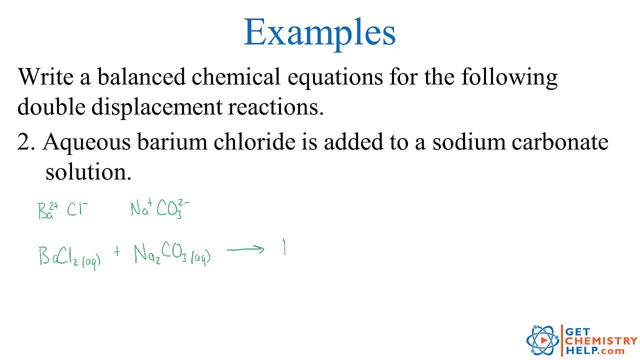 So barium partners up with carbonate. Barium carbonate would be BaCO3.. And if you look on your solubility rules and find carbonate ion, all carbonates are solid, except for lithium, sodium, potassium, ammonium. That's not any of these. 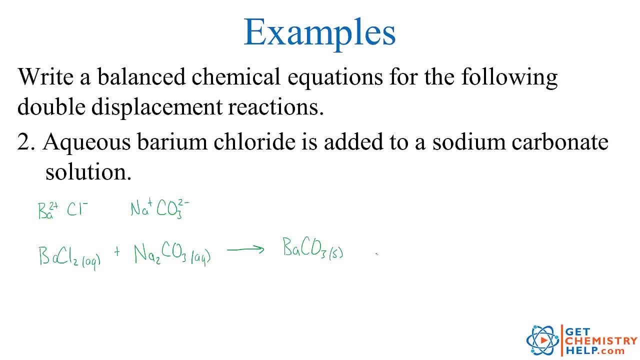 So this would be a solid, And then sodium: It would partner up with chloride So that would make NaCl And all sodium containing compounds are soluble, So this would also be aqueous. So our last step would be to balance this. 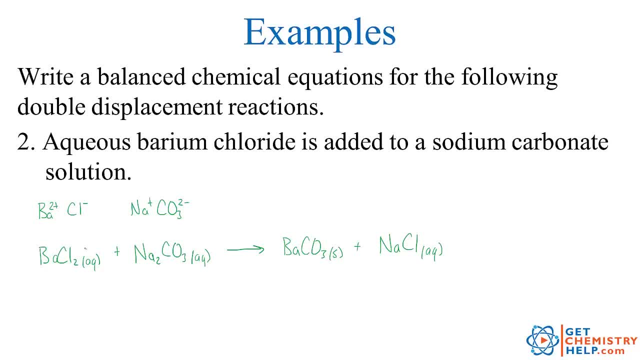 So one barium on the reactants, One barium on the products, Two chlorides on the reactants, One on the products. We need to make that two. Well, now, that also makes two sodiums on the products And we have two sodiums on the reactants.